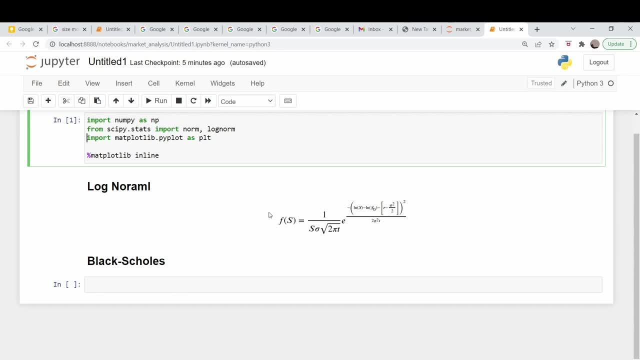 But we're just going to use the built-in statistical functions. We're going to brute force it with this equation here, And then we're going to use the built-in statistics function, Probably normed, because forcing this to be used Usually the long-norm function- is actually a bit of a pain. 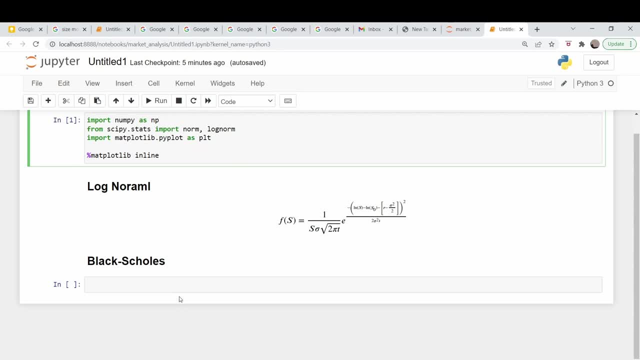 So we're going to use the built-in functions to do it, And then we're going to use the Black-Scholes model And we should get the same number because Black-Scholes is based on this assumption here. So let me come up here and I'm going to insert a line below here: 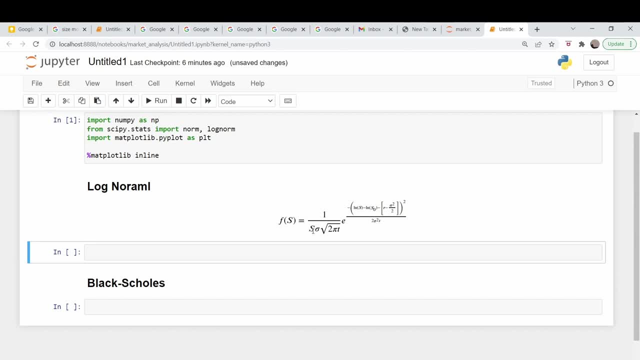 So in this equation here, S is the price of the stock that we're interested in. So this is going to be our variable of interest. Sigma is the volatility, and I'm going to assume implied volatility, And I prefer that rather than any sort of historical volatility, because it's a tradable number. 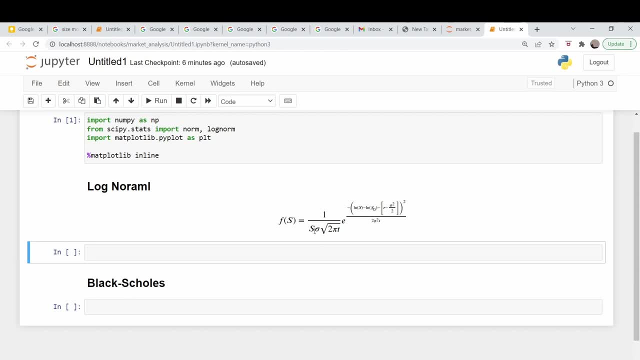 It's a forward-looking volatility. So I think that's the best choice. And the only other variable here- S0, is the initial price of the stock. So if we're interested in, say, the price of a stock closing between $100 and $120,. 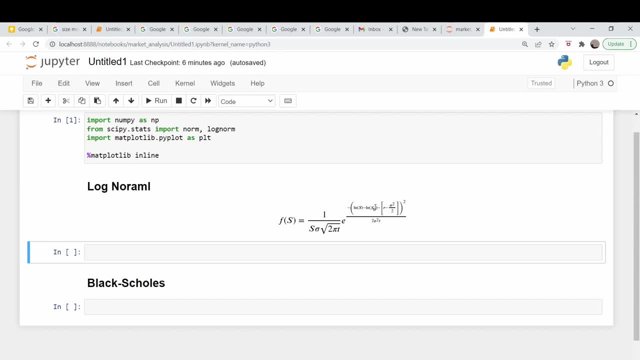 S0 would be our initial price, Assuming the stock started at that price, And S would be that range of prices from $100 to- what did I say? $120.. R is the risk-free rate here And, of course, T down here is time. 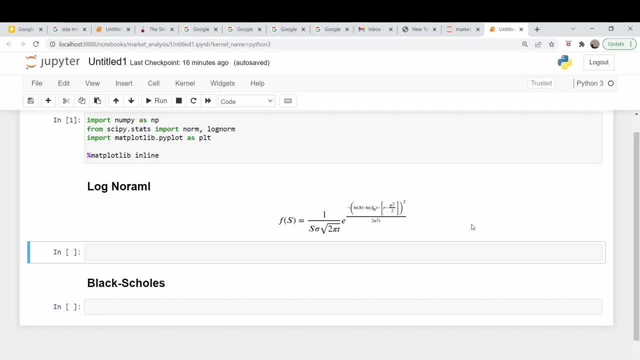 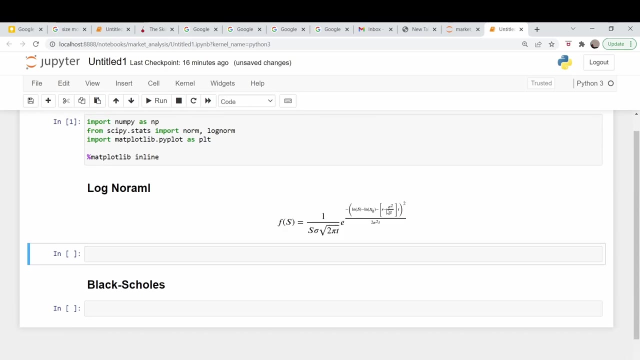 And why does this look funny? There needs to be a T. This term here needs to be a T. It needs to be multiplied by T to make the units work out correctly. So let me do that. Okay, so that's now correct, because T times a rate has to be a price. 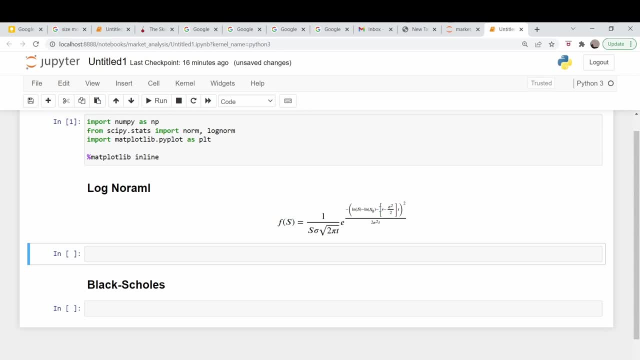 So this has to be price, price, price. So rate times time is price, And then, of course, the volatility squared times time is also a price. So let's just plot this out. Let's assume our S0, what did I say was $100. 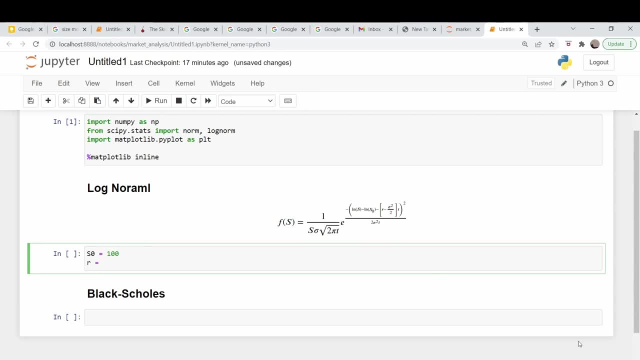 Let's take the risk-free rate, And this is the number we actually don't know. Volatility is a tradable number, so we can get a good ballpark of that just from option-implied volatility. But risk-free rate or the actual drift rate here the risk-free rate we know. 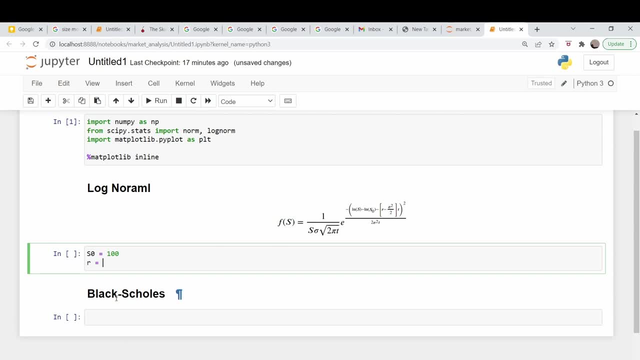 But the drift rate we assume to be the risk-free rate, which is, you know, it's an assumption. So let's take time to be one year And sigma to be I don't know. Let's take it to be 25%. 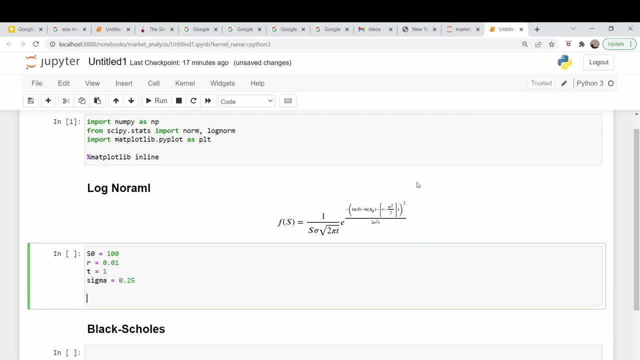 So does that look right? Good, I'm going to write a function now to implement this equation here, And I'm going to do it in a cell above this, one Cell Insert. So here's our function. It just takes the arguments here: stock price, initial price rate, volatility and time. 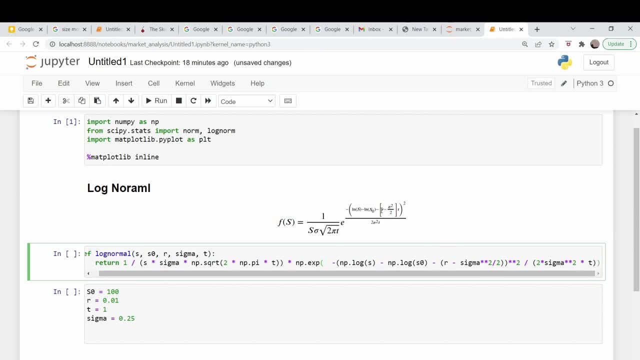 And it just returns this equation right here. So let's just plot, Run that cell And let's plot this out. Let's take our stock price from I don't know: Let's go from 80.. NPlin space: Let's go from 80 to 150.. 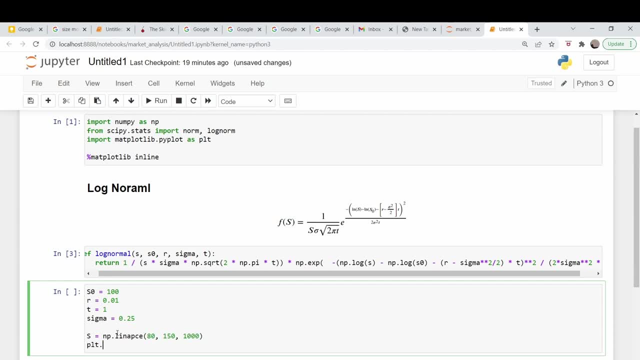 Let's do a high density of points, So 1,000.. And then PLTplot S, And then our function log norm S, S0.. R Sig Can't spell sigma today, Sigma And T, And we'll just make this a solid black line. 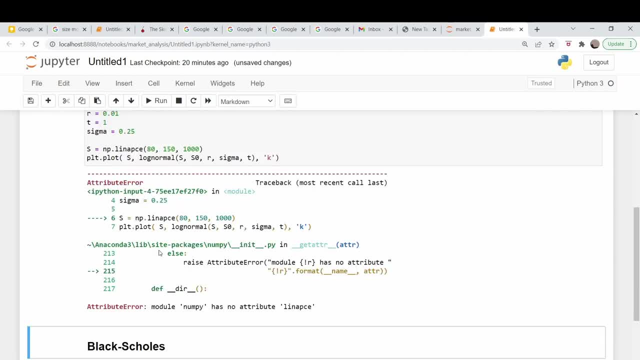 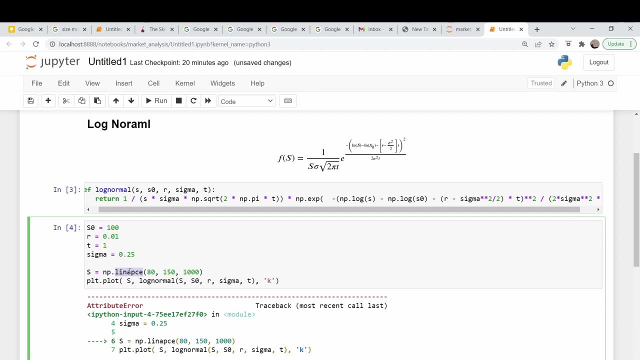 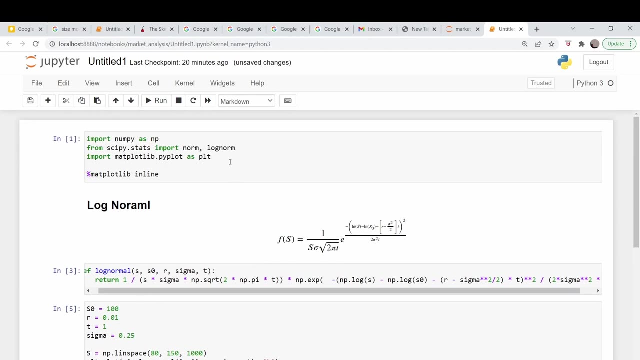 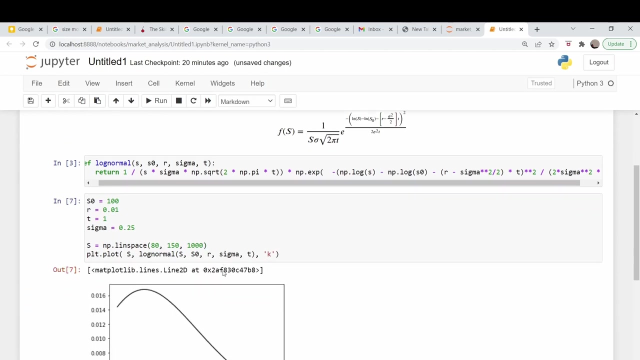 Of course there's an issue: Lin space, Lin space, Lin space- I forgot Lin space, PLT not defined. Did I not run my imports up here? Run that, Run that. I guess I didn't run my imports. 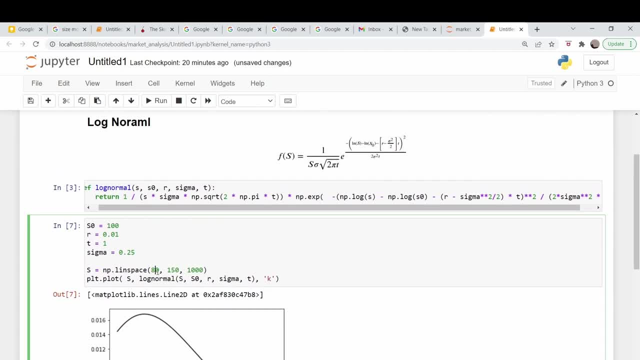 So this is what it looks like. Let's actually extend out the range. Let's go from 50 to 150.. In fact, let's just go- I don't know- 20 to 200.. I just want to actually get a good representation of what this function looks like. 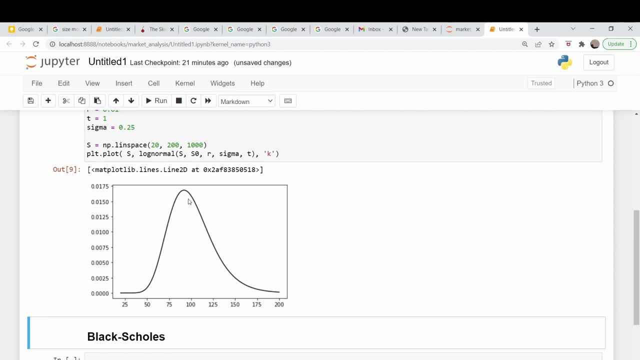 So here it kind of looks almost like a bell. It looks like a bell curve, but it kind of has this fat tail at this, this end, here And now. the way to brute force the probabilities is to pick a range of prices. Say, we believe the stock will be between 100 and 120 and we want to figure out the probabilities. 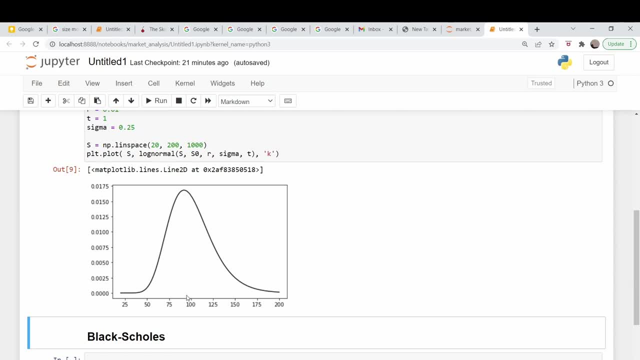 Well, from basic calculus, that's just the integral of this curve. It's the area under this curve between 100 and 120.. So when I upload this to GitHub I'll make a nice pretty picture here with like a shaded area to show that that area. 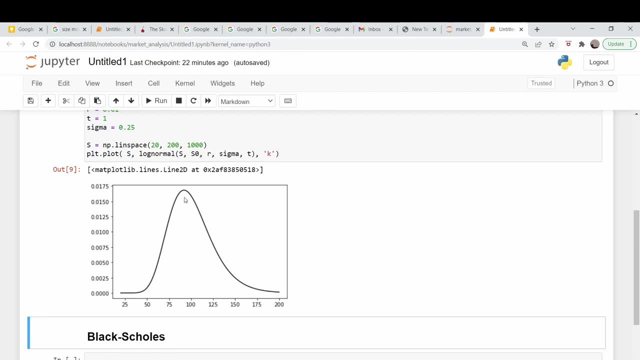 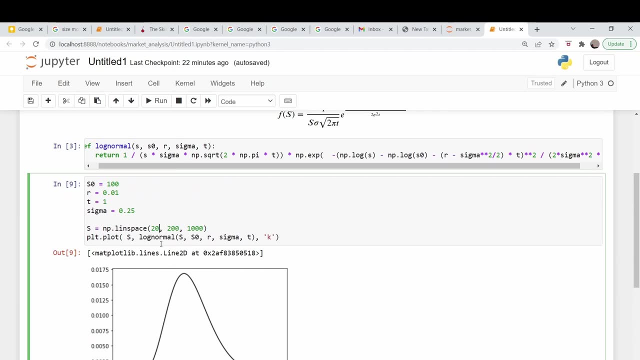 But from basic calculus we just do this, this integral. So in NumPy what you can do is we will set this to the prices we're interested in, say 100, 120.. And I'm not going to plot it anymore. 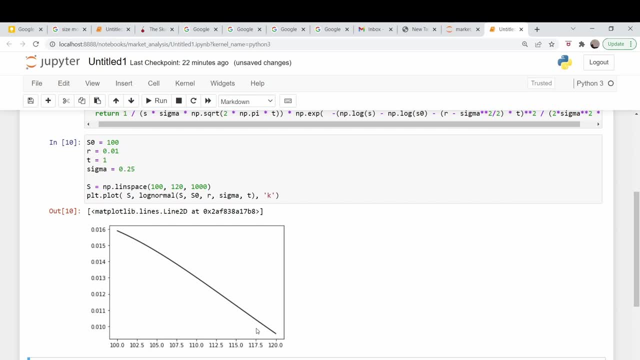 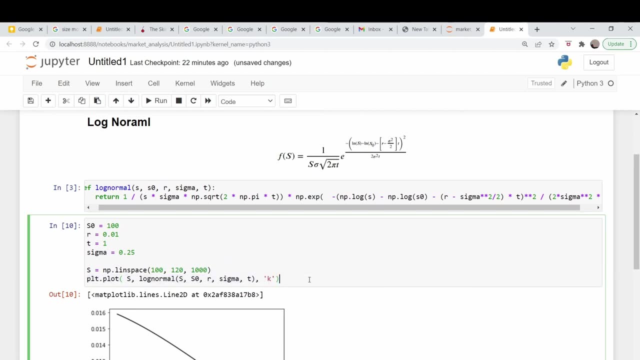 This is the actual area we are interested in here, Almost like a triangle, because this isn't very super, super steep curve here. So let us just comment Out the plot here. NumPy is simple Numerical integral function is called TrapZ. 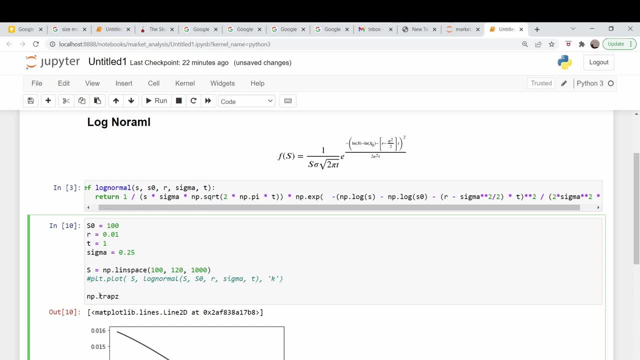 So NPTrapZ is a trapezoidal method to approximate integrals. We do our variable that we're interested in our Y variable. So that's this here, this log, normal thing. Let me just copy and paste it. And this is the opposite of MATLAB. 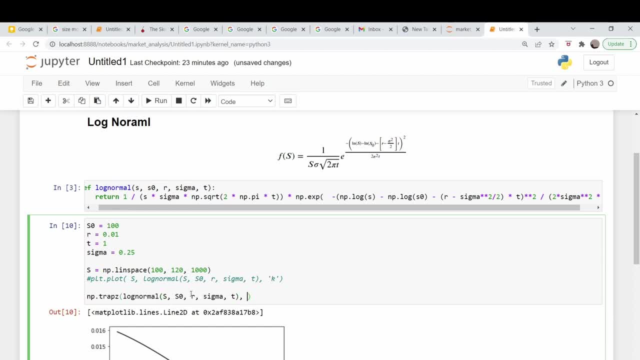 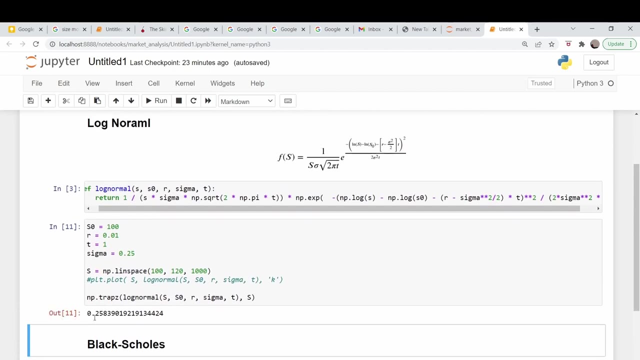 MATLAB does X comma Y NumPy, for whatever reason. does Y comma X, So our X values. here are our stock prices and that's our probability. So in the next year the probability that we will be between 100 and 120, is this number right here? 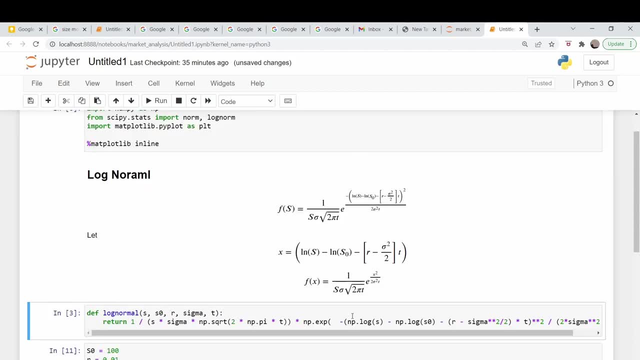 So about 26 percent. So I was going to show a way to kind of recast this in a way that you could use the normal What's it called The series, The CDF, the cumulative distribution function, by recasting this monstrosity here like this and getting an equation like this: 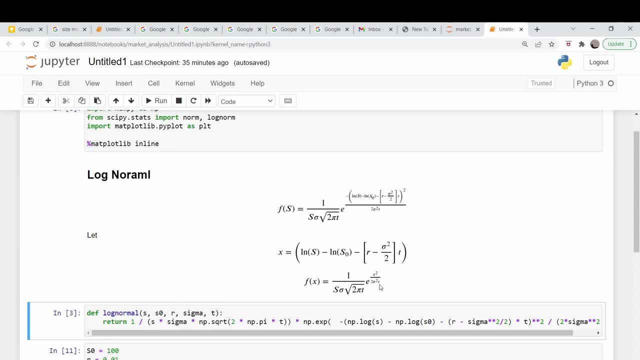 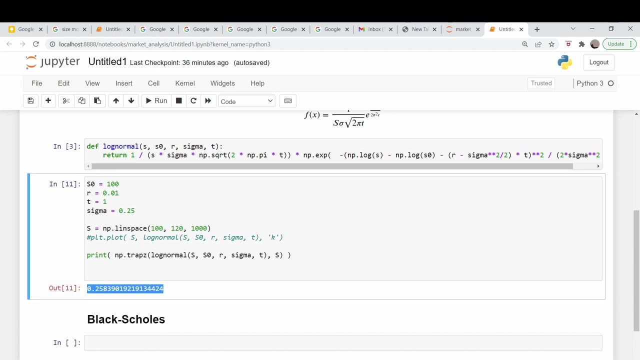 But I forgot that there's this S down here. So when you do the integral, this is not just the cumulative distribution of the normal function, because this S contributes to the integral too. So scratch this This part is probably the correct way to do it. 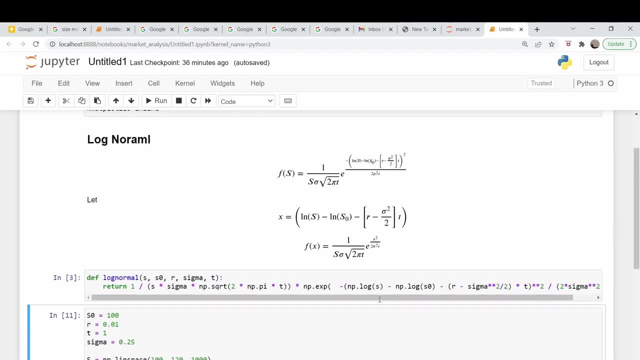 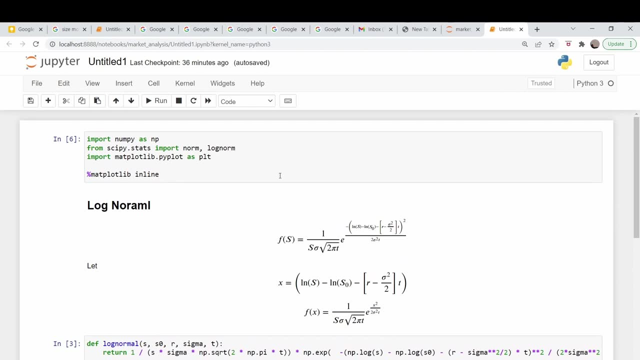 When I upload this, or probably not initially, but eventually I will find a way to recast this to use the built in function. Where is it up here, The log norm, PDF or CDF? The issue is this kind of screws it up. 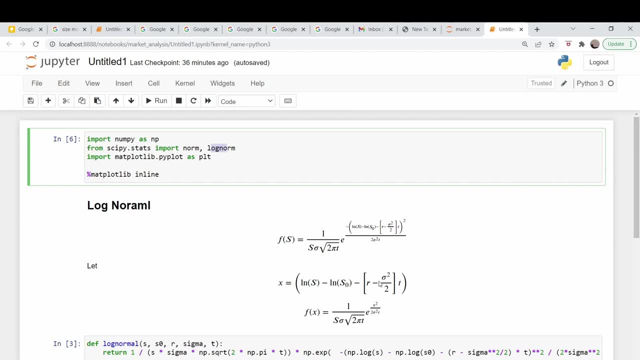 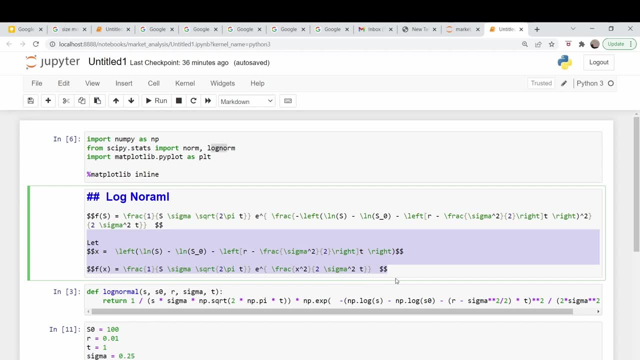 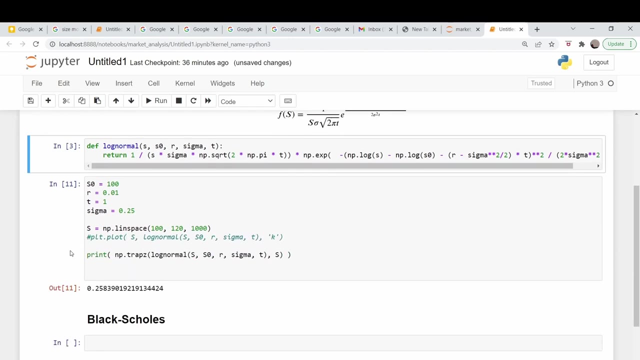 This term screws up the form that it goes into the the this equation, And so, anyways, I'll worry about that later. 3. Let's just do the same thing using the Black- Scholz model, and hopefully we get the same answer as here. 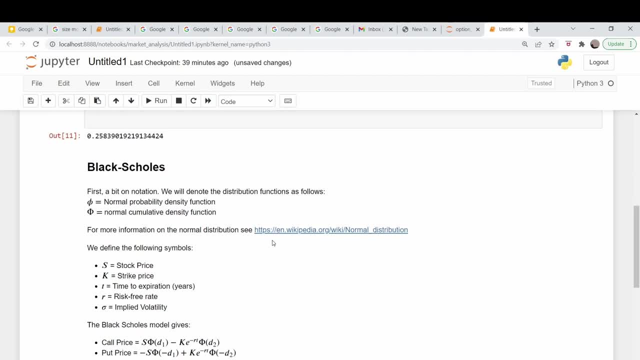 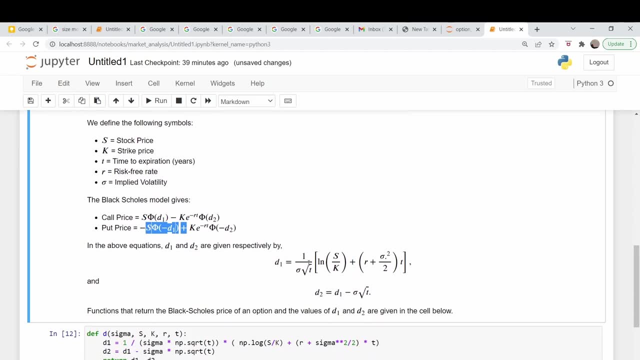 So I copied this from a video we did on the Option Greeks. It's just the equations for the Black- Scholz model: price of a call, price of a put. And we're going to be interested in these D Values, D, particularly D2.. 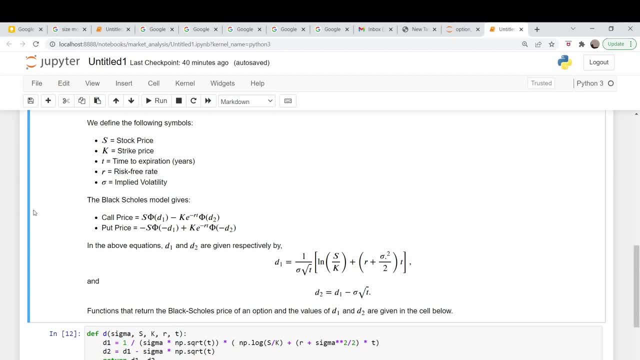 So the probability of a call expiring in the money with a strike price of K is just given by the cumulative distribution function value precisely for theミ, Definitely, is just given by the cumulative distribution function evaluated at D2.. So I copied a function that we had written some time ago to calculate both D1 and D2.. 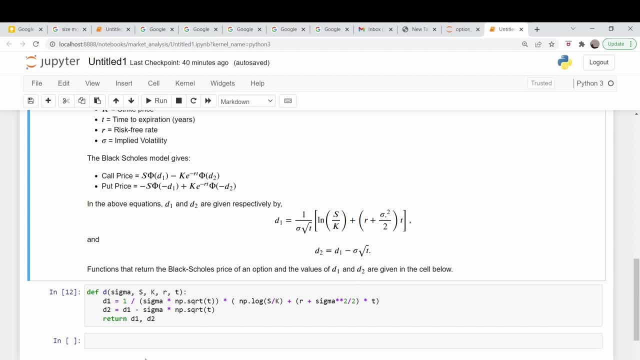 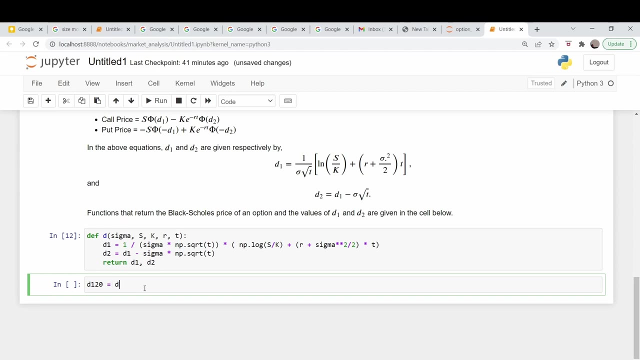 So we are going to just use this and hopefully we will get the same answer or at least do a numerical rounding error as this. So let's calculate our D2 value for 120 first. This is going to be equal to our D function sigma. 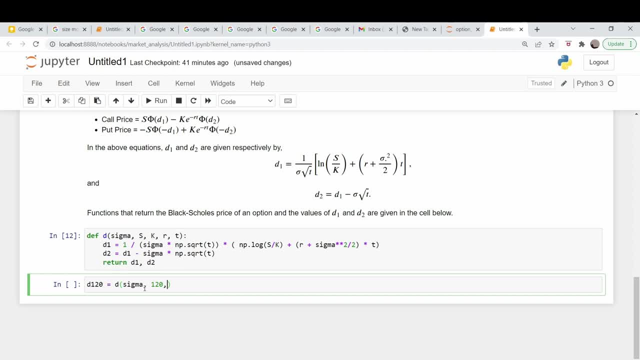 Our stock price is going to be 120.. Our strike price is also 120.. Actually, our stock price is 100.. It's the starting stock price. 120 is our strike price, R is our risk-free rate and T, of course, is T. 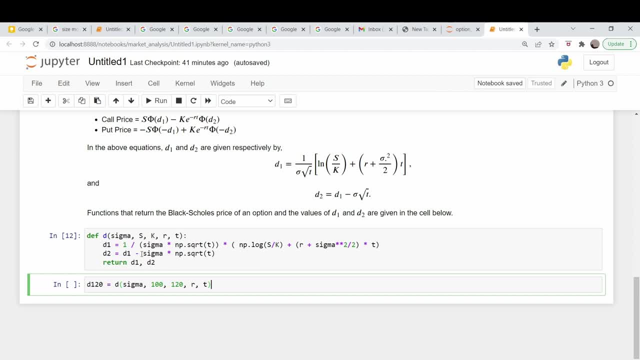 And this returns a tuple in the second variable and that tuple is our D2 value. So I'm just going to do that. I'm going to do D1.. Let me print it out to make sure it's actually calculating it: D120.. 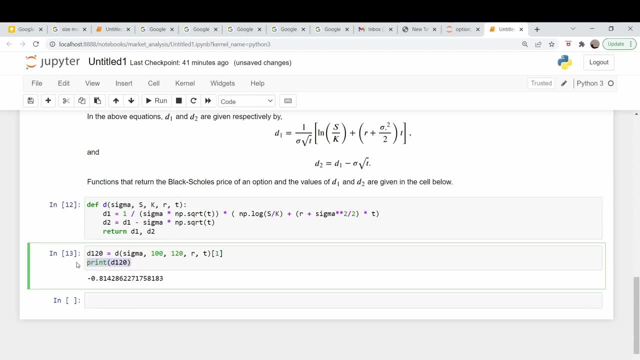 Yeah, cool. So let's do the same thing for D100.. So I'm just going to copy this, paste this: Our new strike price is 100.. And that seems to run okay. So our probability should just be Normcdf D100, minus normcdf of D120..